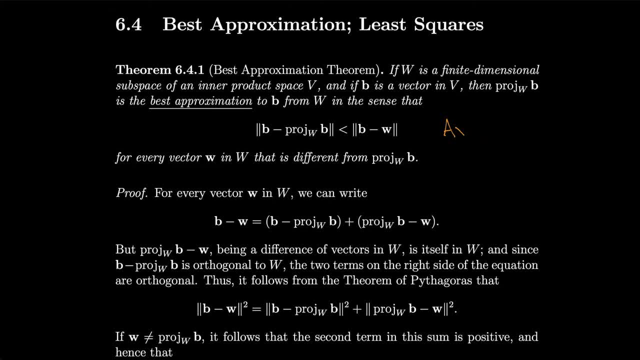 which tells us that the smallest vector x should be b minus the projection of b onto w for b minus w. So let's prove this real quick: for every vector w and w, we can write b minus w as b minus the projection of b onto w plus. 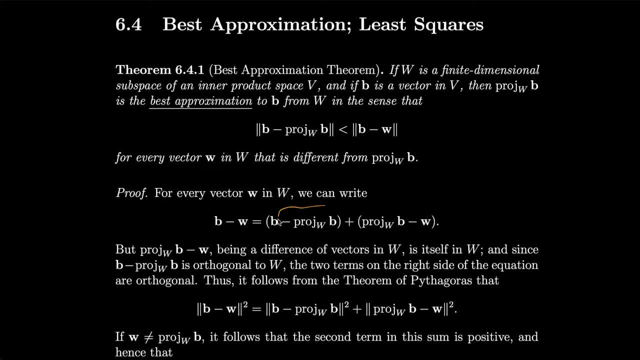 a projection of b onto w minus w. So we're just subtracting and adding this vector right over here and that's the same thing as just adding zero, so it doesn't change it. this is still b minus w, But the projection of b into w minus w, being a difference of vectors in w, is itself in w. 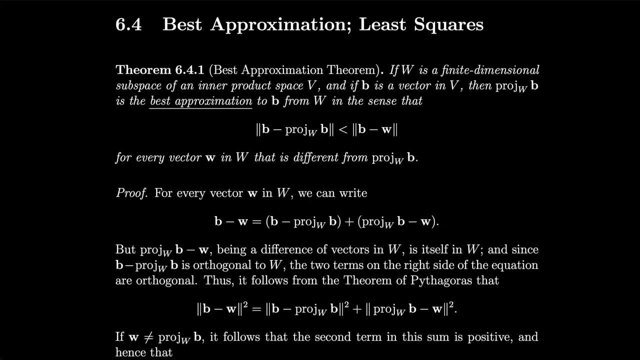 and since b minus projection of b into w is orthogonal to w, the two terms in the right side of the equation are orthogonal. Thus it follows from the theorem of Pythagoras that length of b minus w squared is equal to b minus projection of b into w, squared plus. 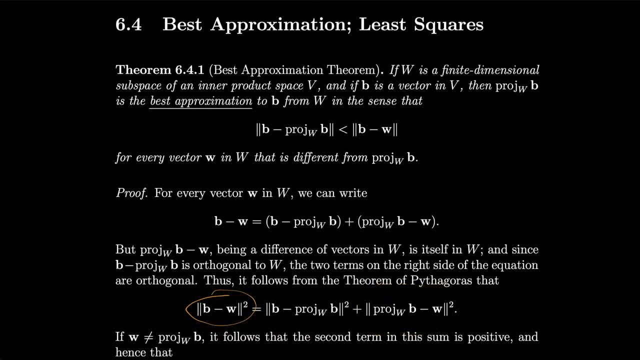 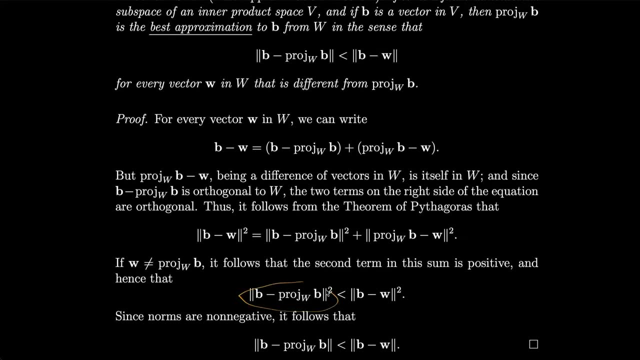 or plus projection of b into w minus w squared. So if w is not equal to the projection of b of w, it follows the second term. this sum must be positive, so that has to be positive and hence that b minus projection of b of w squared must be. 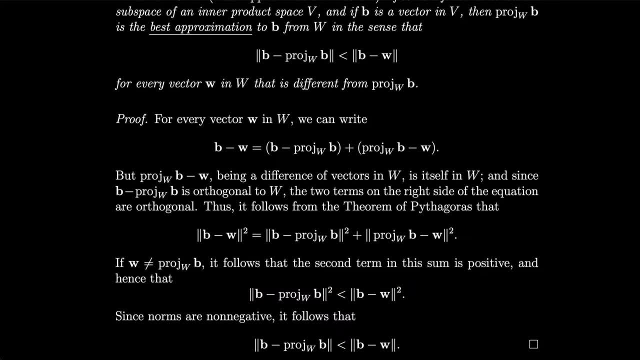 less than the length of b minus w squared. So if this is positive, then what we have left must be less than that. Since norms are not a negative, it follows that we can take the, we can get rid of the square, we can basically take the square root of each one, so we get that the length of the projection of 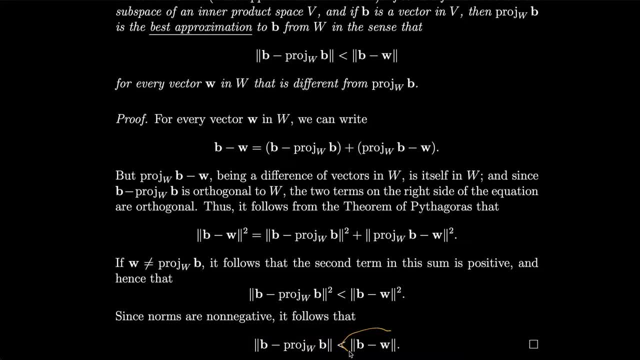 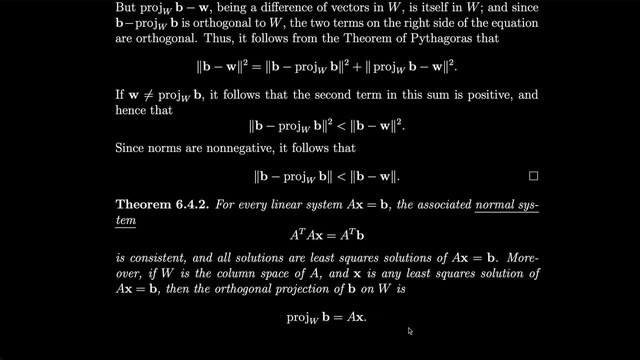 the length of b minus projection of b into w must be strictly less than the length of b minus w. For every linear system ax equals b, the associated normal system- a transpose ax equals, a transpose b- is consistent and all solutions are least-constrained. So if a is the least-square solution of ax equals b, then a is the least-square solution of ax equals b. 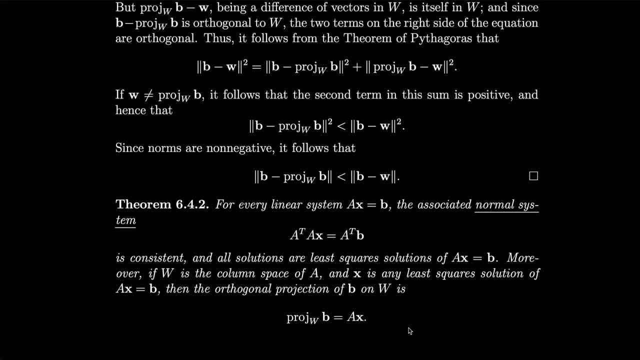 Moreover, if w is the column space of a and x, is any least-square solution of ax equals b? then the orthogonal projection of b on w is projection of b on w equals ax. So we're basically saying that we're going to come up with a least-square solution. 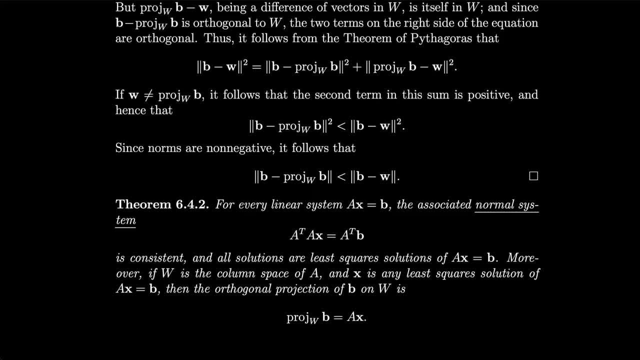 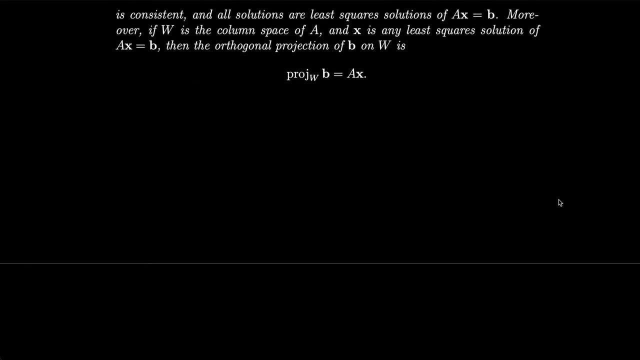 in other words, an approximate solution to the system, in the sense that we can now figure out approximate solutions for inconsistent systems. that's really the motivation here, And we're going to take advantage of the previous theorem in order to do that. So let's do an example real quick. we'll find the least-square solution. we'll find the 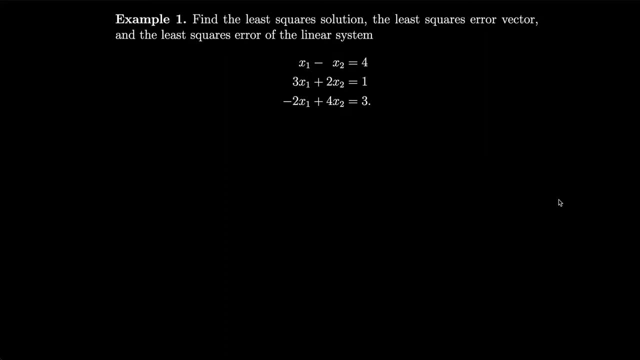 least squares error vector and the least squares error of the linear system given. So first we'll write out: ax equals b, So a is just the coefficients. so one minus one, three, two minus two, four and b is four one, three. So let's look at a transpose a so we can use the previous theorem. so a transpose a is one. 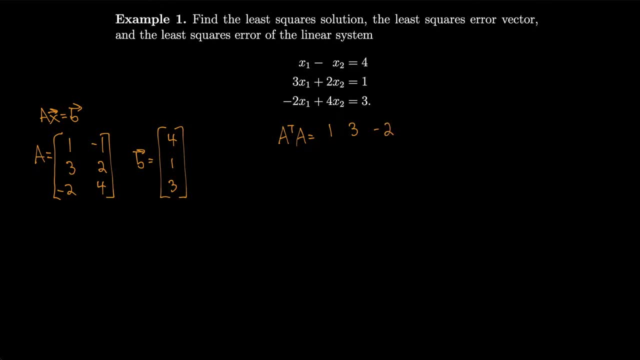 three minus two. just take that column, make it into a row, and minus one, two, 4, multiplied by a, which is 1, 3, minus 2, minus 1, 2, 4.. So, doing the multiplication, we get 14, minus 3, minus 3, 21.. 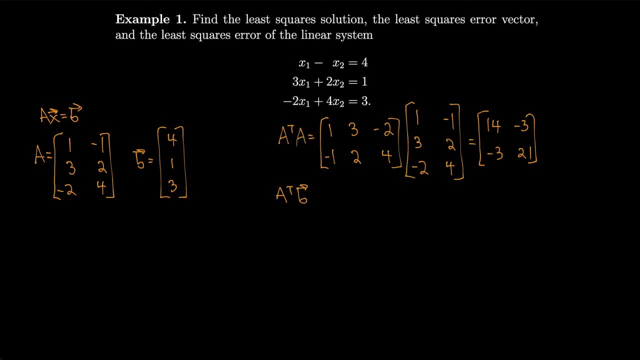 Let's get a transpose b now. So that's 1, 3, minus 2, minus 1,, 2, 4, multiplied by b, which is 4,, 1,, 3, and we get 1, 10.. 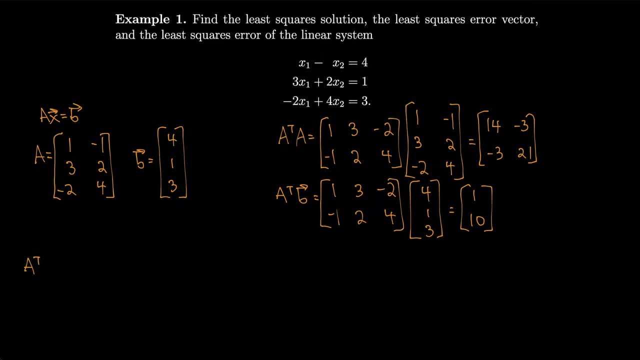 Okay, so now let's write out the equation: a transpose ax equals a transpose b, So that's 14, minus 3, minus 3,, 21, times. how about for x? we make it x1,, x2.. 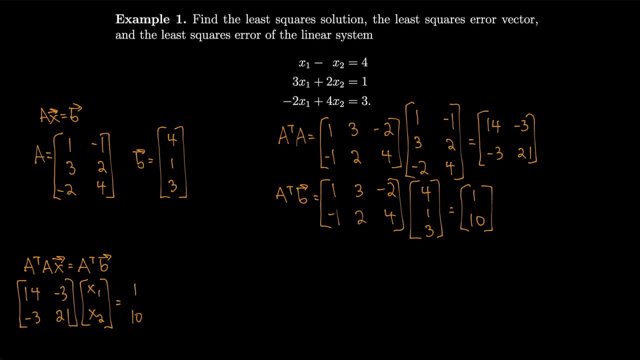 And we'll set that equal to a transpose b, which we computed as 1, 10.. So then let's see if we can solve this system. How about i? I divide the first row by 14,, so I'll get 1, minus 3, over 14,, and this 1, I'll adjoin. 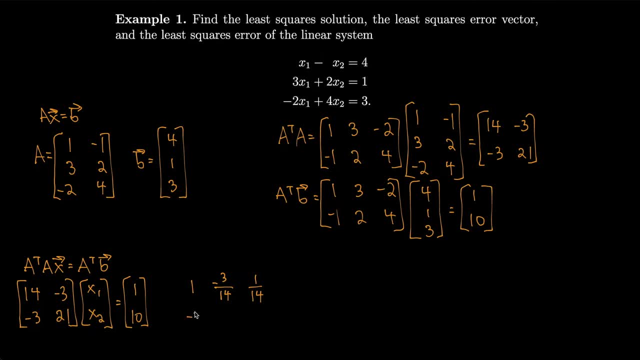 so I'll get 1 over 14, and then I'll keep the second row minus 3,, 21,, 10.. Okay, let's keep going and let's get a 0 underneath. so I'll keep the first row 1,. 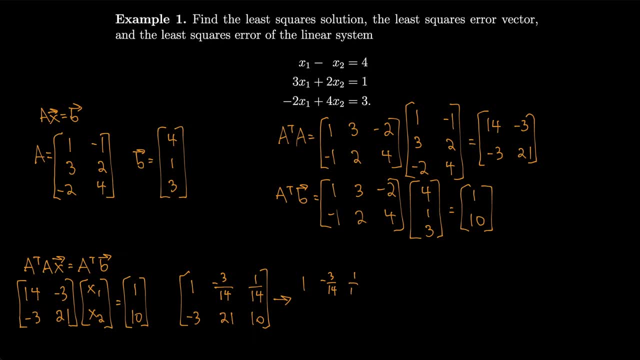 minus 3, over 14, 1, over 14,. but for the second row I'll subtract 3 times the first or I'll add 3 times the first and I'll get 0, 285, over 14, 143, over 14.. 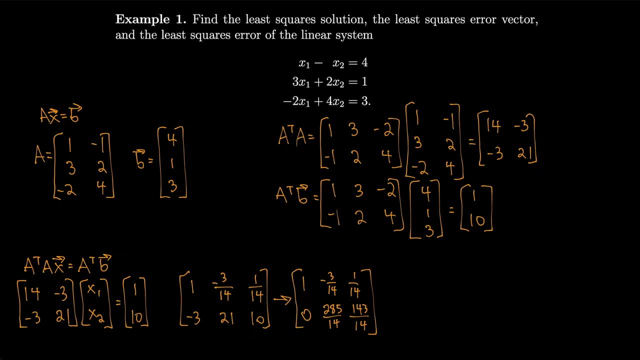 And then I'll multiply this row by this reciprocal in order to get a 1 over there. so I'll get the same top row, 1, minus 3, over 14, 1, over 14, but for the bottom row I'll get 0, 1, 143, over 285.. 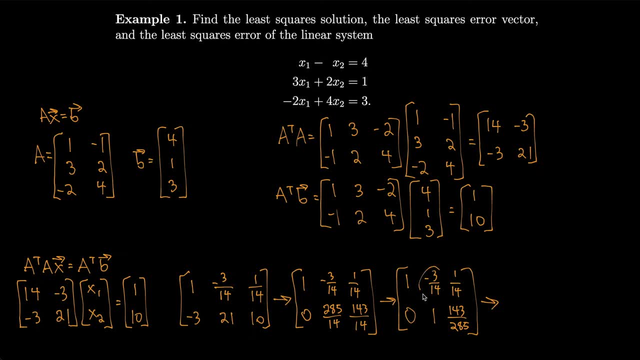 Then I'll keep going and I'll get a 0 above that 1,. so I'll just add 3 fourteenths times the bottom row. I'll get 1, 0, 17, over 95.. And then 0, 1, 143, over 285.. 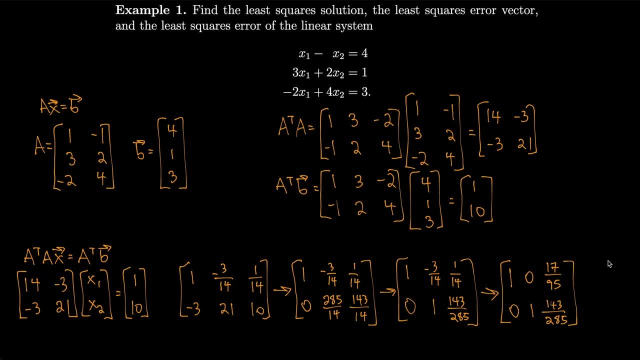 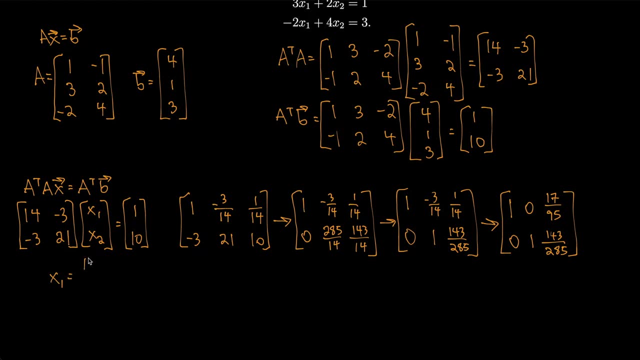 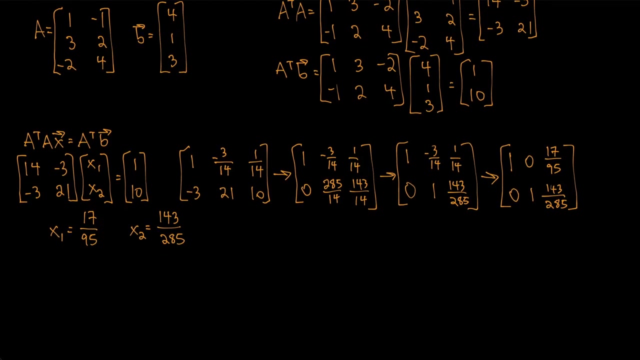 Okay, so now we've solved. ATAX equals A. transpose B, so we see that X1 is equal to 17, over 95, and X2 is equal to 143, over 95.. 285, so now we can approximate B minus AX, so we have: B minus AX is equal to 4,. 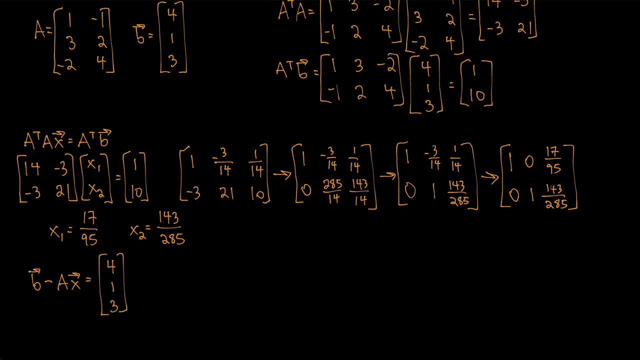 3, minus 1,, 3, minus 2, minus 1, 2, 4.. for a: and then we're plugging in this x, which is 17 over 95, 143 over 285, and that equals- let's simplify a little bit- 413 minus minus 92 over 285. 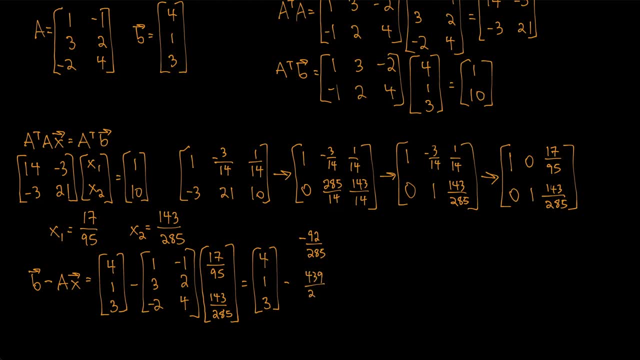 439 over 285 and 94 over 57, and then, subtracting, we get 1232 over 285 minus 154 over 285 and 77 over 57. so all we need to do is get the length of that and we have our approximation. 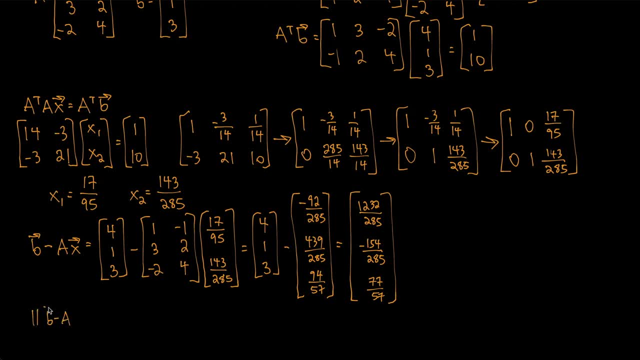 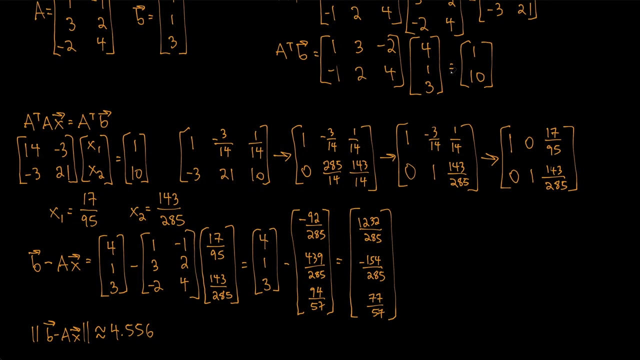 so that means the length of b minus ax. if we take the square root of each of these squared, add them up so we get approximately 4.556. so we found the least squares solution. our least squares solution was what we got from over here, where we had x1 equals 17 over 95 and x2 is 143 over 25. 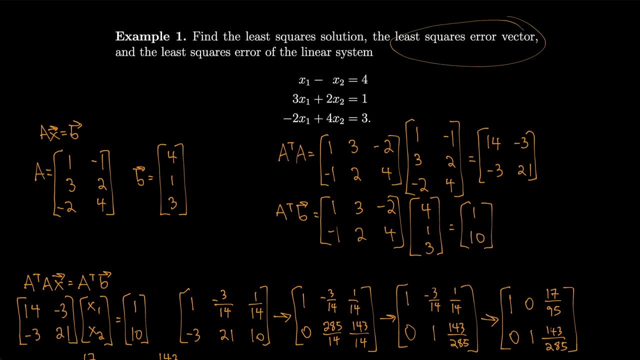 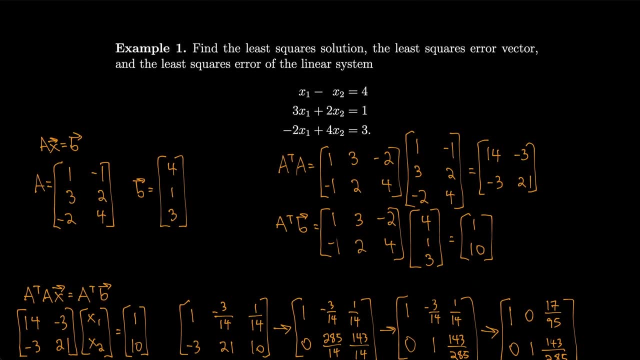 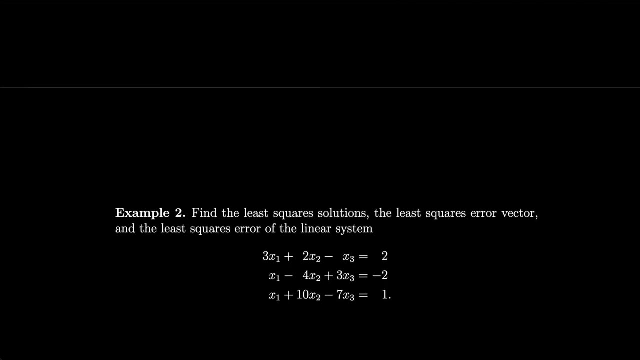 we found the least squares error vector. that was b minus ax, that's equal to this guy. and then we found the least squares error. that was the last thing we did, by just finding the length of the least squares error vector. how about we do another example? let's find the least square solutions least. 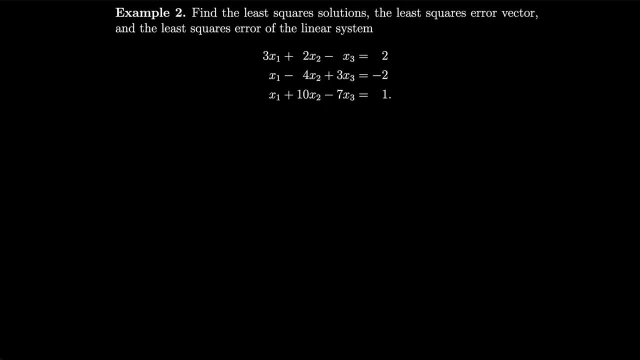 squares error vector and least squares error of this linear system now. so again we'll write out: ax equals b. so in this case we have a equal to 3, 2 minus 1, 1 minus 4, 3, 1, 10 minus 7, and we have b equal to 2, 3 minus 3, 1. let's look at l A. transpose a. 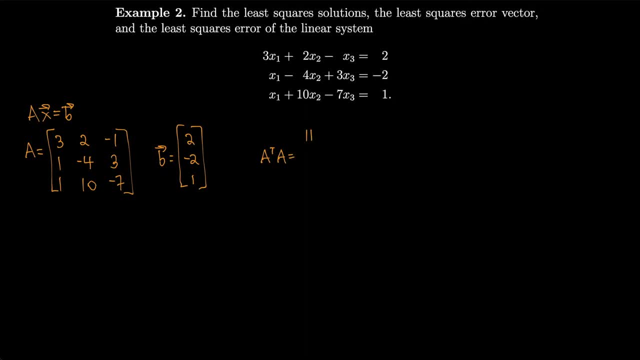 11, 12 minus 7, 12, 1, 20 minus 84 minus 7, 12, 120 minus 84, 384, 121, 2, 187, 188, Nestle plus 182, 286, 286, 10 to the power of 2 out of 188 minus 8. 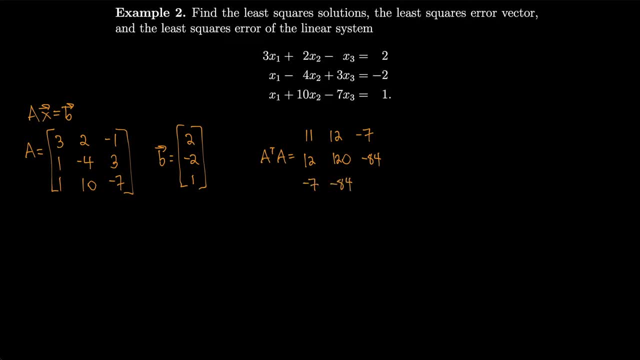 288 minus 386, 87 minus 84, 59. if you do the multiplication a, transpose b. if you do that multiplication, i'm not gonna do it for you- is 5, 22 minus 15. sorry, but i'll just run out of space. then let's do a. 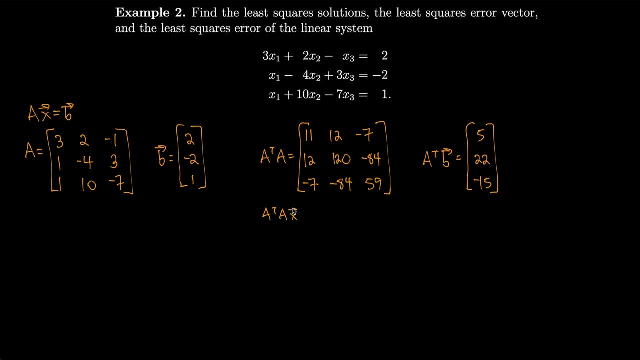 transpose a, x equals a, transpose b, so we get 11, 12 minus 7, 12, 120 minus 84 minus 7 minus 84, 59, and i'll join that with 5, 22 minus 15 and i'll solve that system. 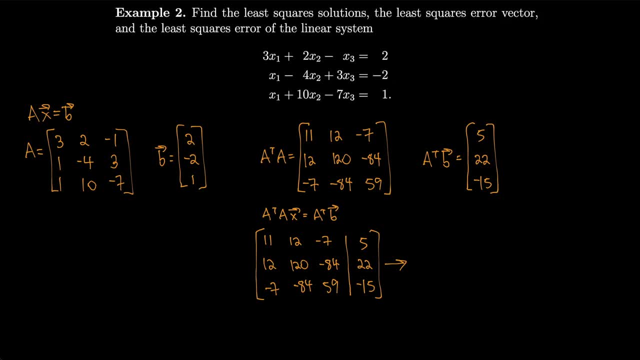 so what we can do is, uh, subtract off, divide, do basically the same thing we did last time. it turns out that the reduced row echelon form will end up being one zero one seventh, two sevenths, zero, one minus five sevenths, 13 over 84, and the last row becomes all zero. 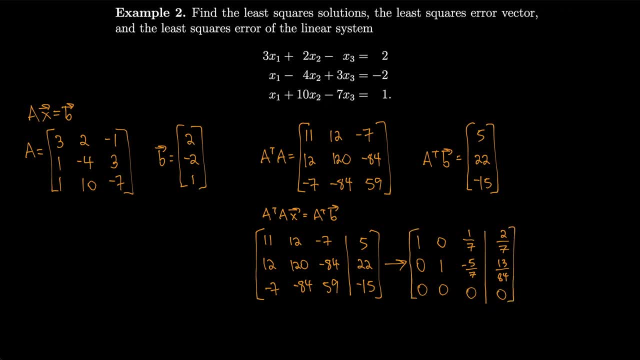 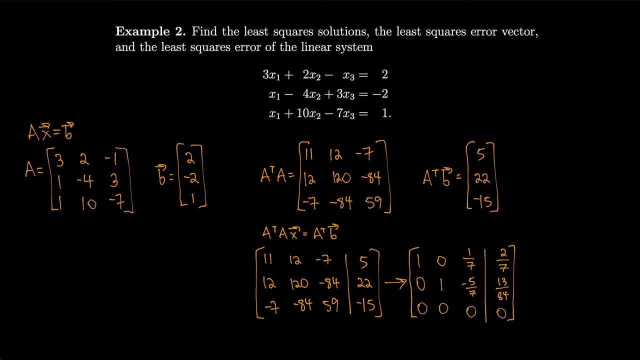 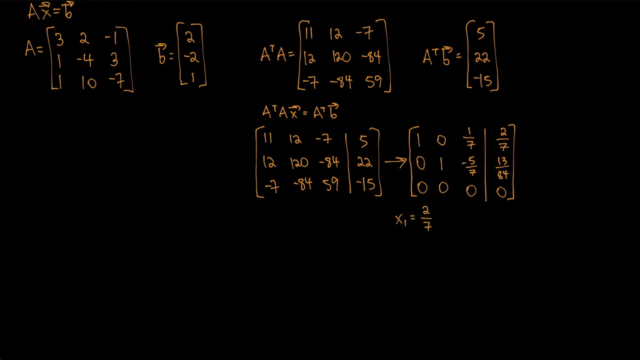 it just takes a little while to reduce it, or you could use a calculator. in any case, we see that for our least squares solution, we get: x: 1 equals 2, 7 minus 1, 7 t. x 2 equals 13 over 84 plus 5, 7 t, and that means that x3 is our parameter t. 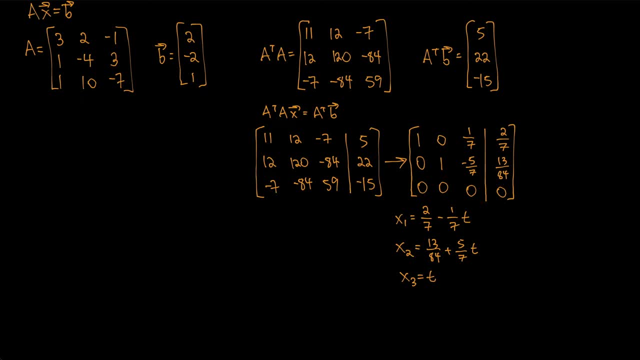 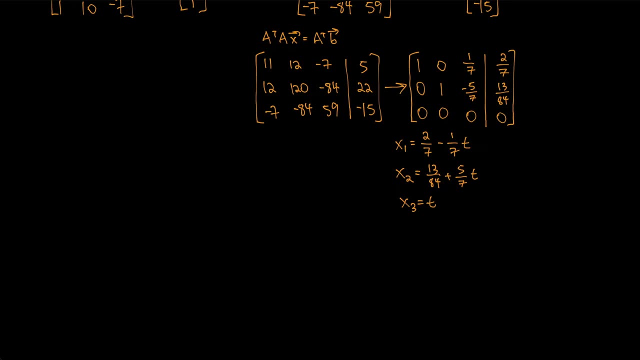 just from that third row of zeros. so we have our least squares solution. let's find out how far off it is. but let's look at our least squares error vector. so we have our least squares error vector. so that's b minus a x, which equals 2 minus 2, 1. 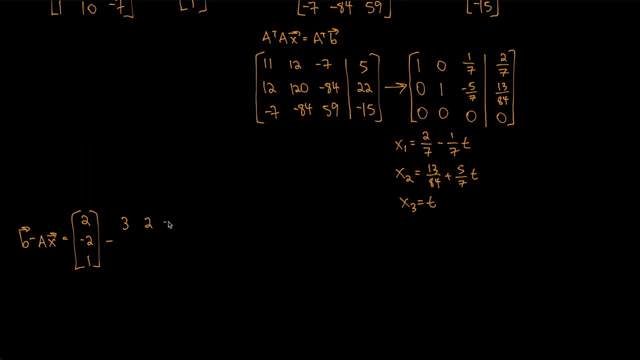 minus 3, 2 minus 1, 1 minus 4, 3, 1, 10 minus 7 times times 2, 7 minus 1, 7 t, 13 over 84 plus 5, 7, t and t. okay, so simplifying a little more, we get 2 minus 2, 1 minus 7, 6. 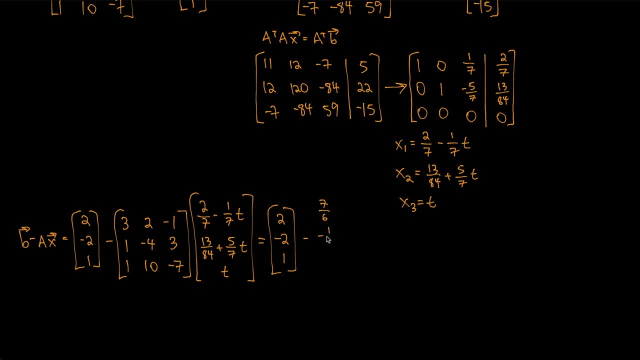 minus 1, 3rd, 11, 6, and that ends up becoming 5, 6 minus 5 thirds minus 5, 6. let's get the error now, now that we have the error vector. so we'll take the length And we get 5: 6 squared plus minus 5, third squared. 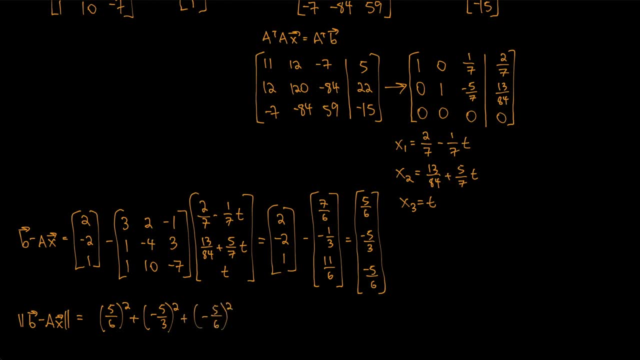 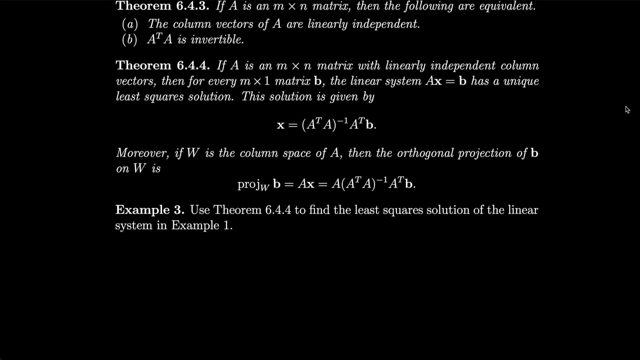 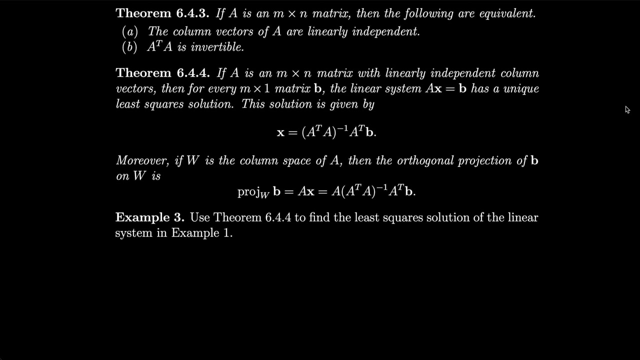 plus minus 5, 6 squared. Take the square root and it equals 5: 6 rad 6.. If A is an n by n matrix, then the following are equivalent: The column vectors of A are linearly independent and A transpose. A is invertible. 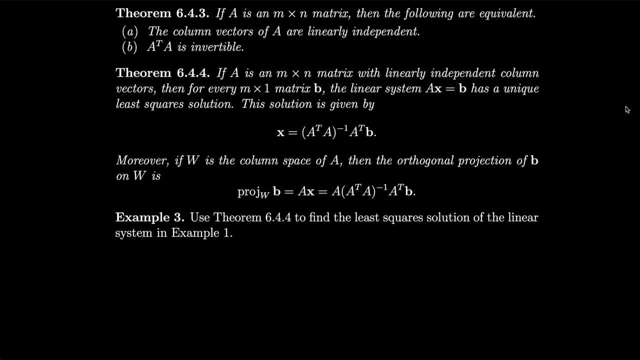 We'll use that theorem but we won't prove it. If A is an n by n matrix with linearly independent column vectors, then for every n by 1 matrix B, the linear system A x equals B has a linear system A x equals B. 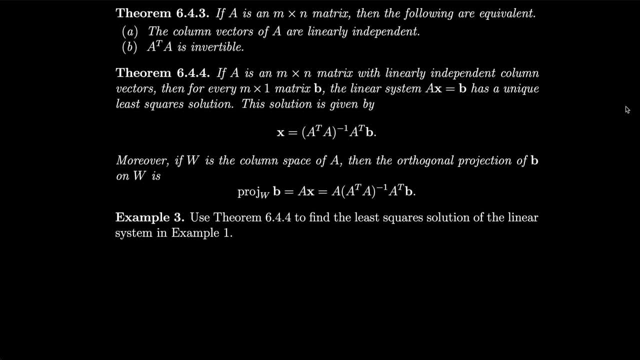 has a unique least-square solution. This solution is given by: x equals A transpose A. inverse A transpose B. Moreover, if W is the column space of A, then the orthogonal projection of B on W is equal to A, x, which is this quantity over here. 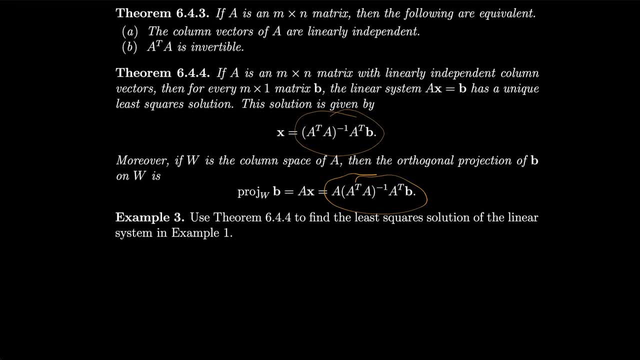 from before: A transpose A, inverse A transpose B. How about we use this theorem now to find the least-square solution of the linear system in example 1.. So what we'll do is we'll write out: x equals A transpose A. inverse A transpose B. 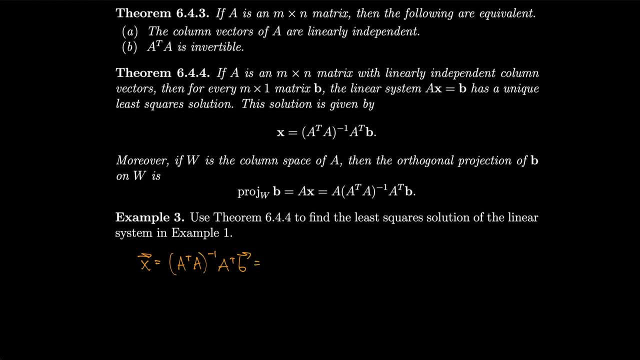 Instead of the least-square solution that we got before. so this is an alternative: we'll do 14 minus 3 minus 3, 21,, and we'll take the inverse of that and we'll multiply that by 1: 3 minus 2 minus 1, 2.. 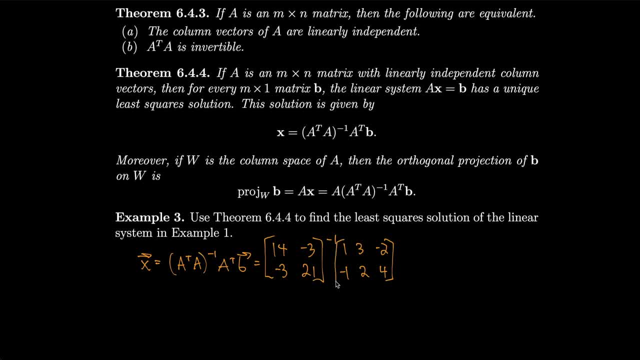 1, 2, 4, and then multiply that by b, which is 4, 1, 3.. Simplifying, we get 1 over 285, 21,, switch with 14, and then minus minus 3 is 3.. 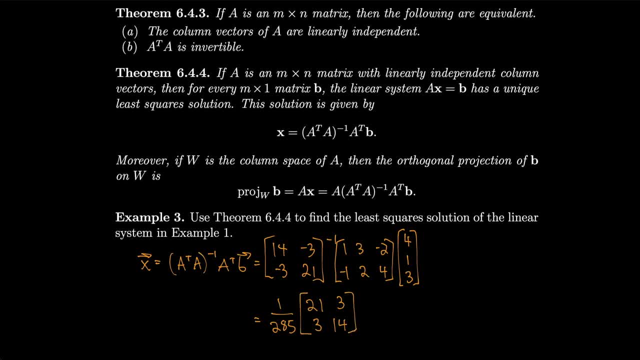 So that's the inverse. and then we multiply that by 1, 3, minus 2, minus 1, 2, 4, and multiply that by b, 4, 1, 3.. Doing all the multiplication, we should get 17 over 95,, 143 over 285.. 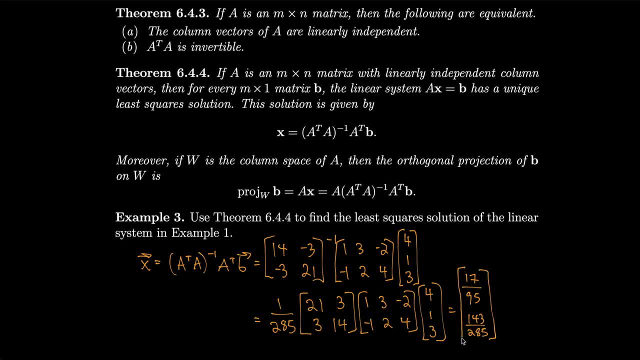 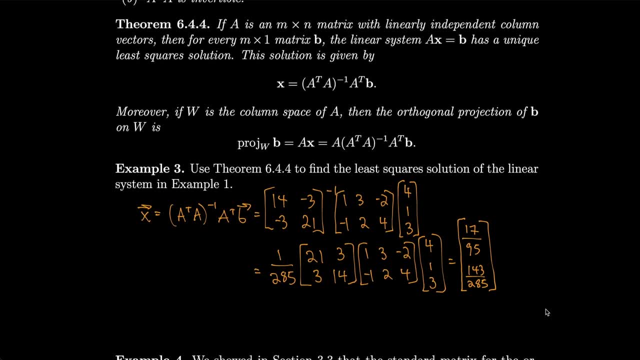 And notice. Notice, that's the exact same least-square solution that we got in example 1, but we didn't end up having to solve any system in order to get it. We just had to do some multiplication. So that's kind of nice. 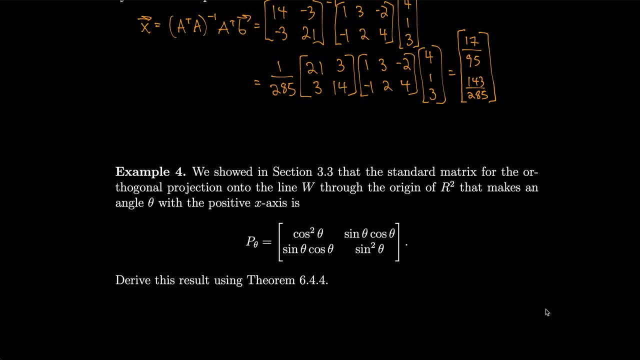 We showed in section 3.3 that the standard matrix for the orthogonal projection onto the line W through the origin of R2 that makes an angle theta with the positive x-axis, is p theta given by this matrix. Let's derive this result using the theorem that we just used. 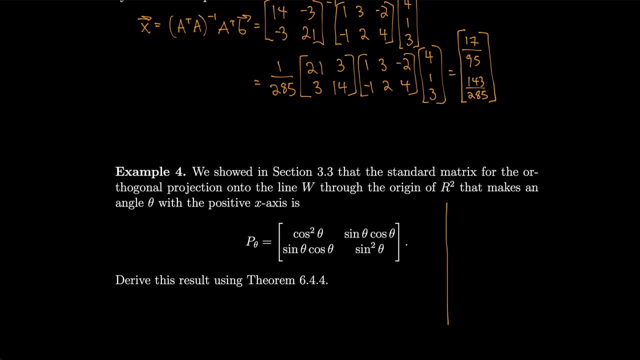 So how about I draw what's going on here? So here would be my y-axis and here would be the x-axis, and we'll put our line W going through the origin, And then we just need some projection onto there through an angle theta, with the positive x-axis. 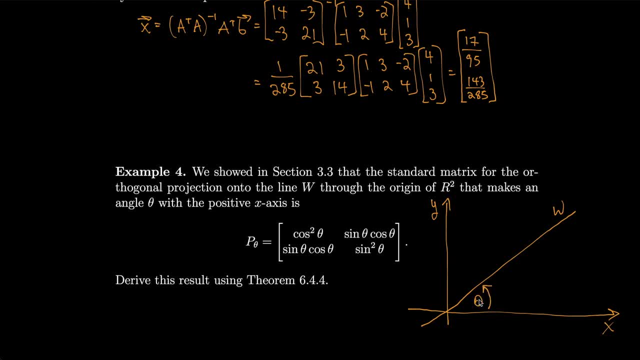 So here will be my angle theta. So I will project onto W. I'll make W the vector with length 1.. So this vector right over here will be W. So that means that the x-coordinate for W, if I go straight down, should just be the cosine of theta. 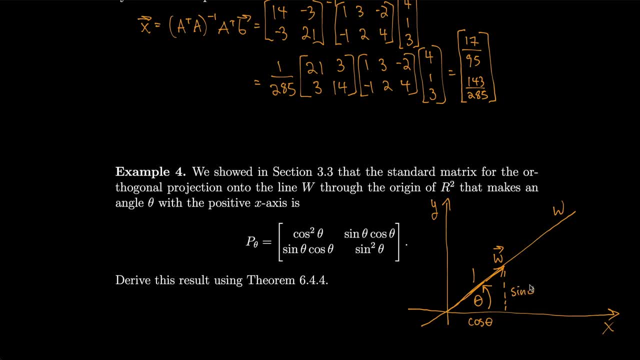 And the y-coordinate for W Should just be the sine of theta. So that means that W has coordinates cosine theta sine theta. So I'll make my matrix A equal to cosine theta sine theta. So now we can compute the least squares solution. 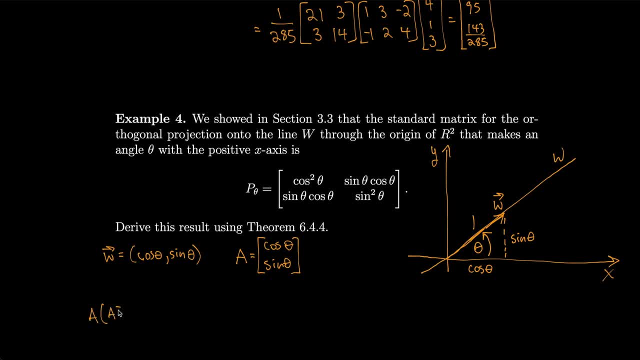 So we'll do A times A transpose, A Inverse, A transpose That'll be equal to cosine theta sine theta. times A transpose, A inverse is actually 1 in this case, And then cosine theta sine theta is A transpose. It's a nice thing about the identities. 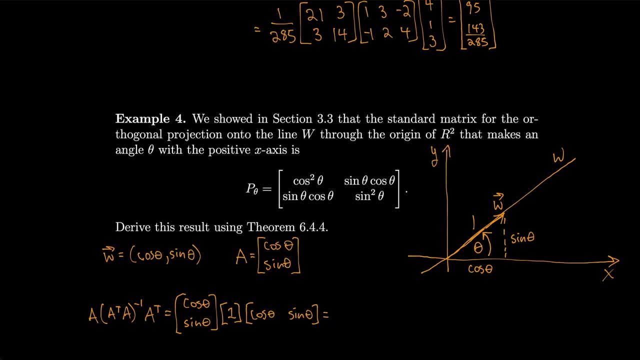 Cosine squared plus sine squared equals 1. Simplify things a lot: Multiplying all this through, we get Cosine squared theta sine theta, cosine theta sine theta, cosine theta and sine squared theta, Which is exactly equal to P theta, as we have previously seen.